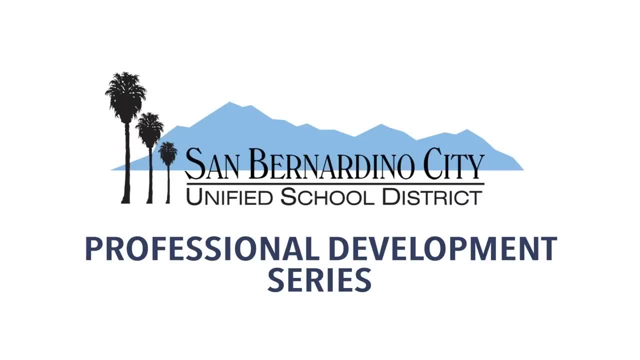 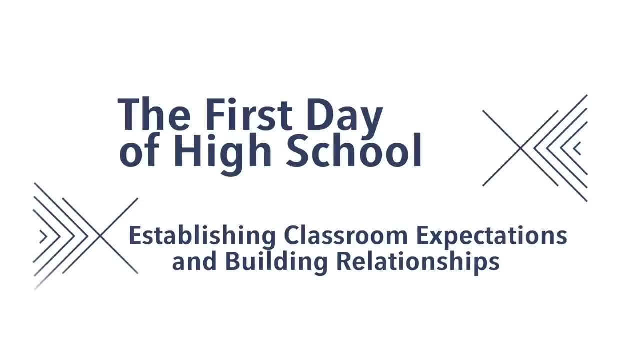 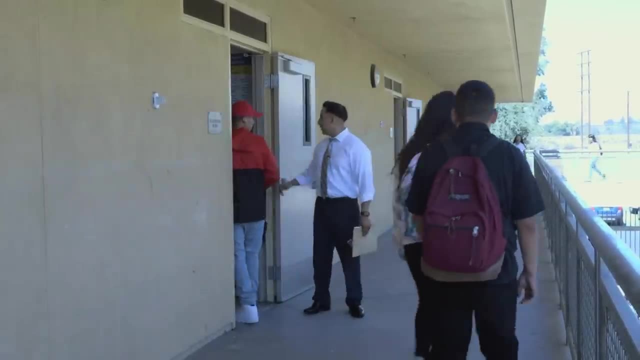 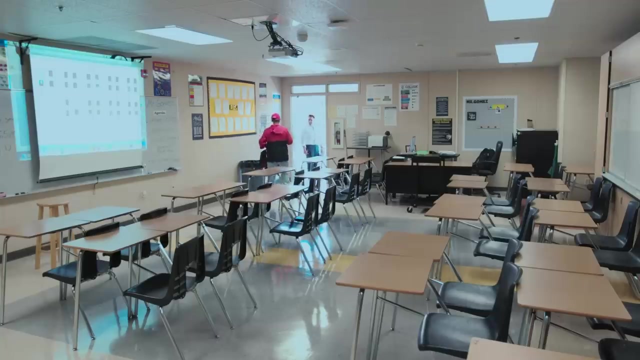 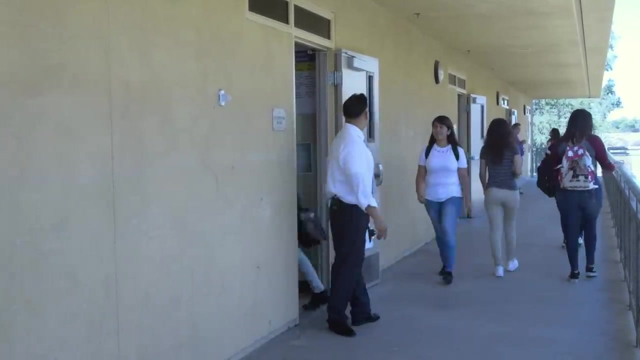 And 203?. Alright, welcome. Find your picture on the board and then there's a number there and then find your seat. okay, Can I see the hat real quick? Okay, Bulls. Okay, But I don't want it in class though. okay, But it's a nice hat though. Hey, welcome Guys, as you guys are. 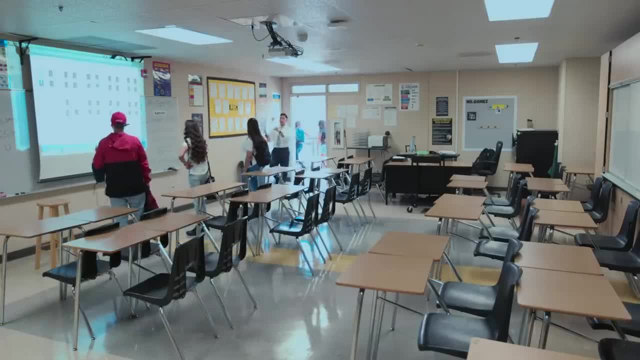 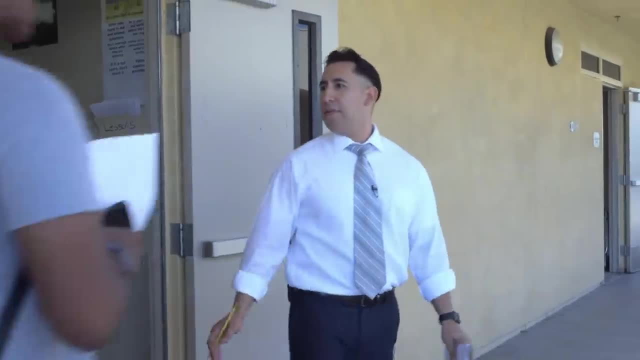 coming in. please make sure that that is you right, And there's a number that's by you and then that's where you guys are going to sit, okay, So that's the seating chart for today. Mr Gomez, Yeah, Alright, welcome, How you doing. 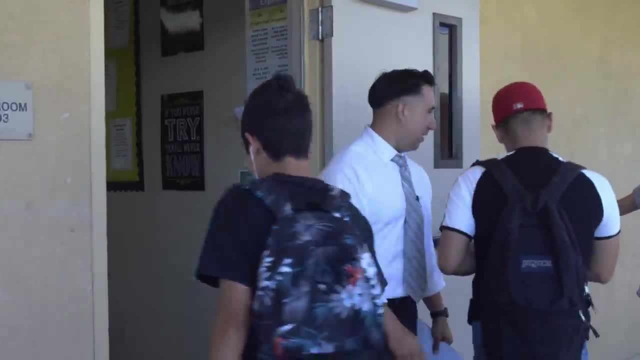 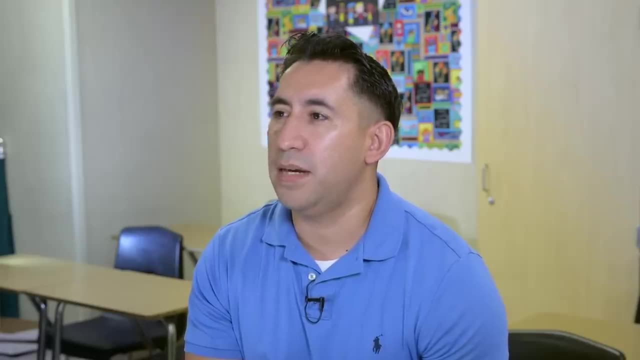 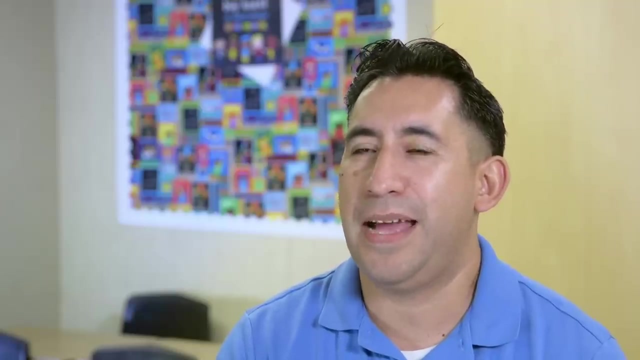 How you doing. Todo bien, Yeah, How we doing. I was outside greeting students. I definitely was out there just trying to establish, build a relationship, because I have never seen some of these students, So to say I really had no. 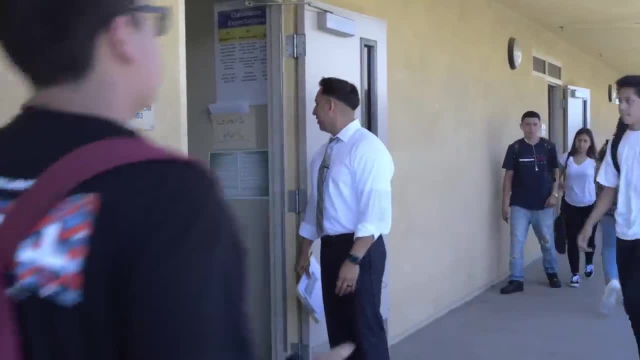 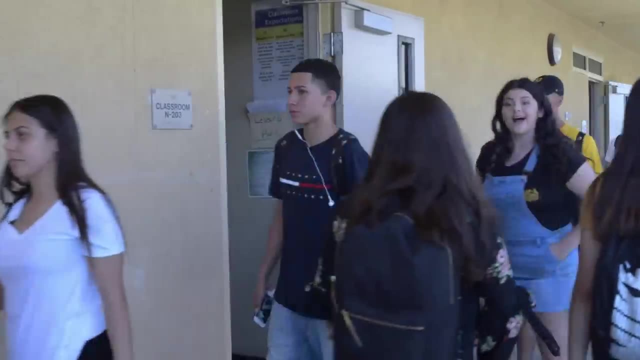 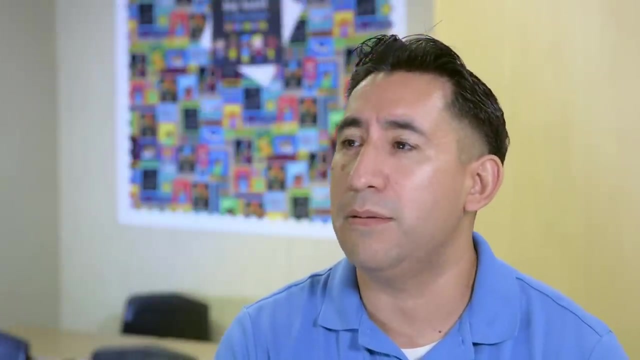 relationship. So I was just trying to find something, whether it was off their shirt, whether it was just something, whether it's just trying to connect with them, even just saying welcome. But I wanted them to feel safe, that this was a place I wanted them to be, and I was happy to be there with them. 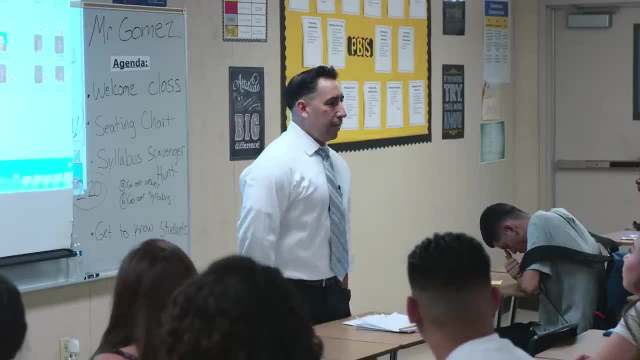 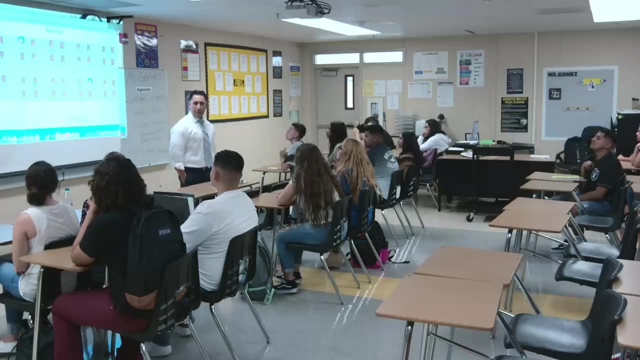 Okay, So real quick. there is a seating chart. okay, Always There has to be. okay, Right, Because it gives structure, Because there's a reason where you're sitting. I made sure that, looking at the math skills, that there's a strong in your group. 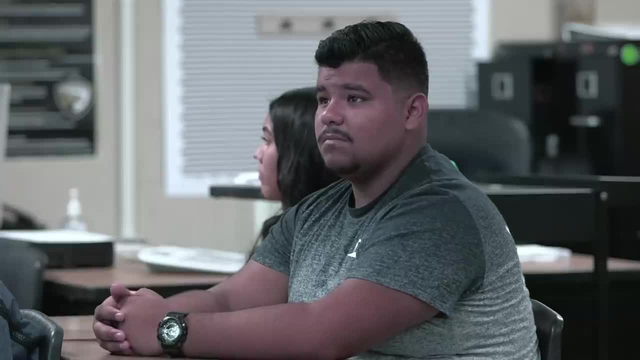 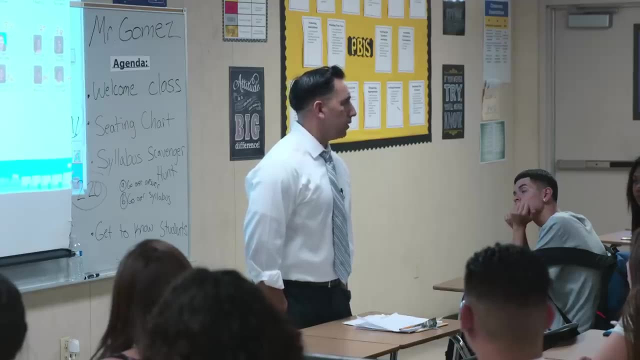 that there's kids that struggle with math- and hopefully my kids that are- that really are strong in their mathematics. it will help you. This is math three, Okay, So it's a little heavier, right, It's a lot more work. 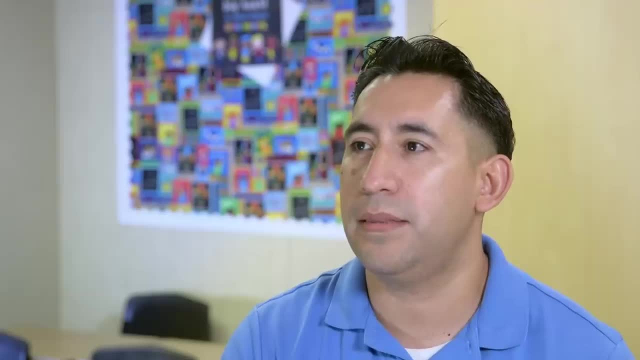 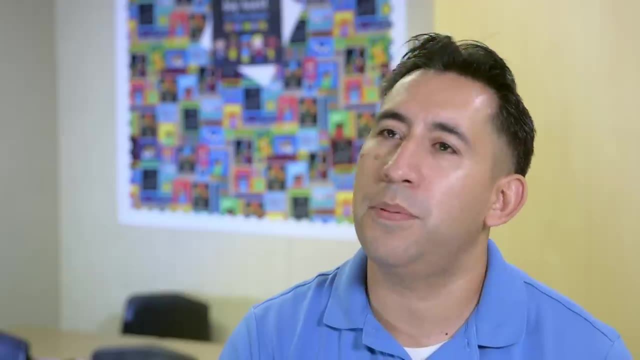 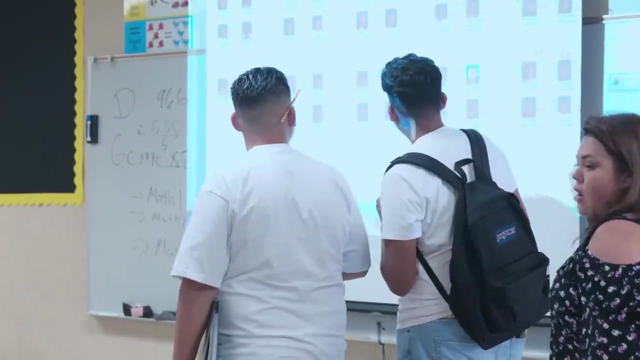 So I had the seating chart set because I noticed that that is day one. I think it gives me more of control. I think it's very important for the students to understand that, even though this is our room, I am still responsible. I'm the main person there that I want to establish this learning environment. 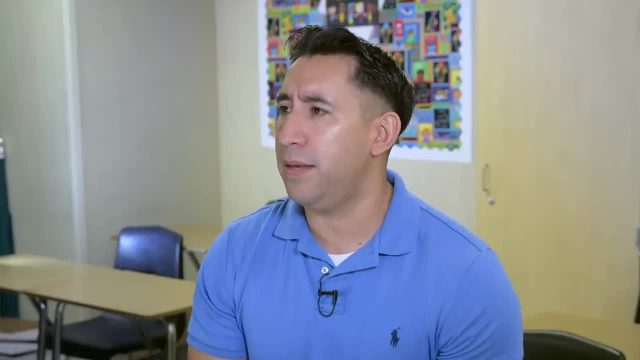 And yes, it shows authority, which is great. Yes, But I think also you're still responsible. But I think also you're still responsible that I didn't just make a seating chart just to make a seating chart. the seating chart was based on levels, was a language, and I noticed as soon as the students 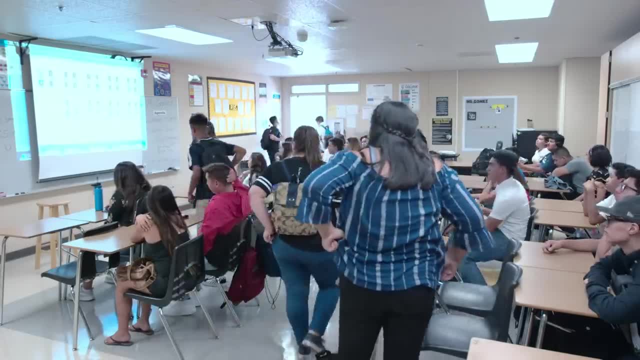 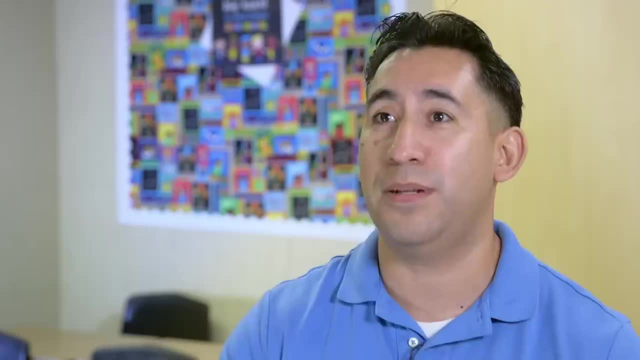 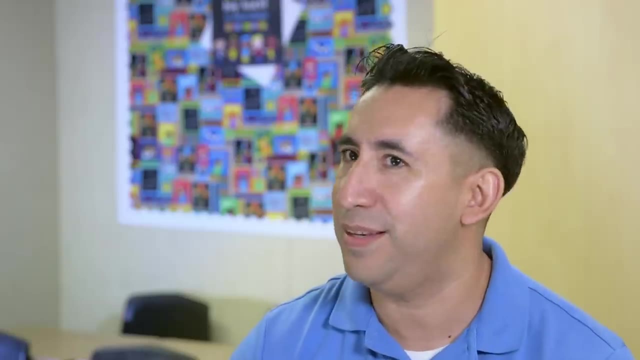 sometimes come really. they come really loud sometimes from the outside to the inside. but as soon as they see the seating chart they actually start to like: wow, this teacher, he actually is in charge or he's authority. I have a feeling he's. he's gonna be addressing the rules now. once again, I want you guys 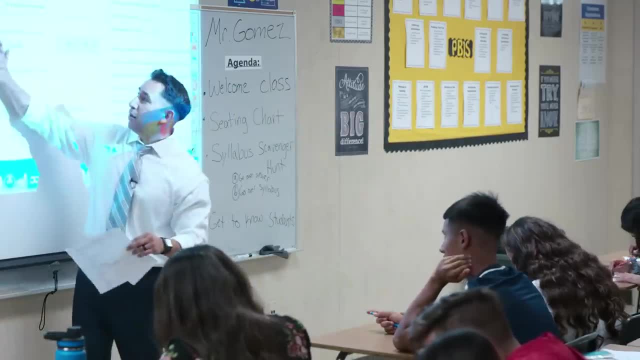 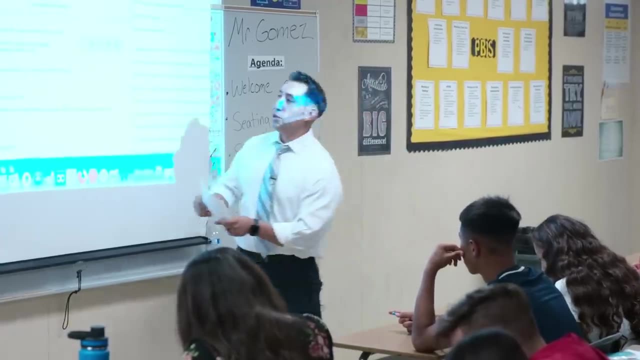 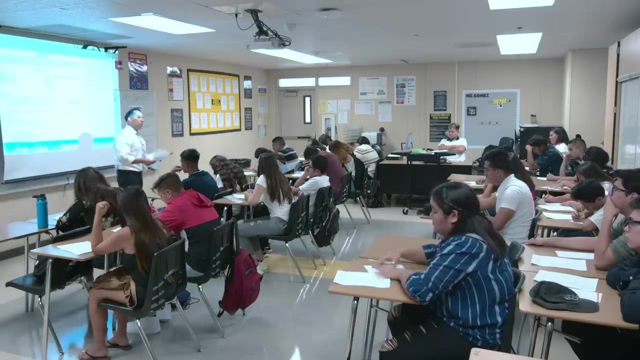 to use this syllabus because that obviously all the answers are here, right, and all you got to do is fill them in. for number one, you can see that it says the first two rules in the class are. you would look where it says rules and then you would start to: yes, right, number one and two and so on. in a little bit I will. 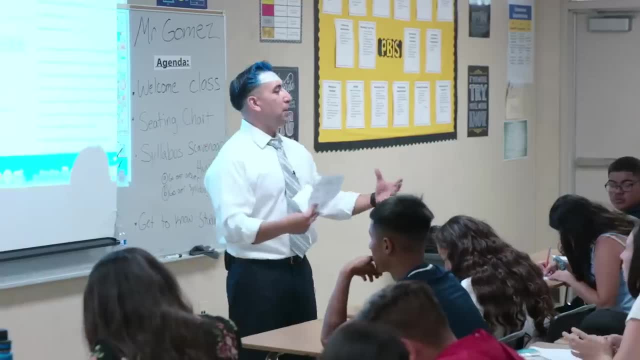 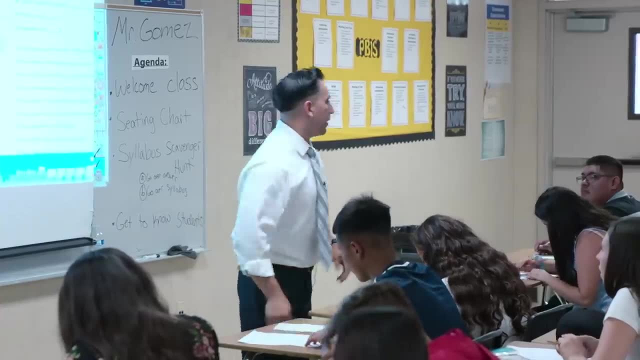 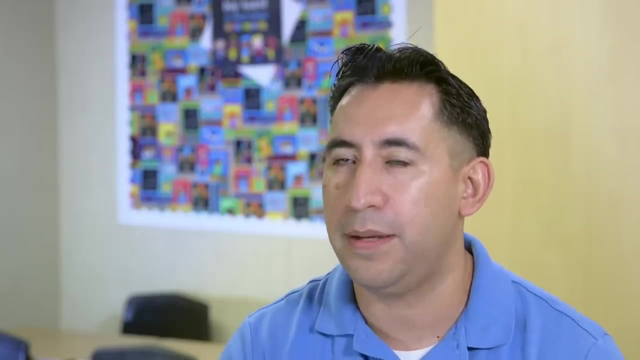 call on your beautiful names and we will hear your answers and then we will make sure that we are definitely having the correct ones. does that make sense? yes, having the syllabus could be very dry could be very boring. most teachers like to have their syllabus on the, on the PowerPoint, and the kids are 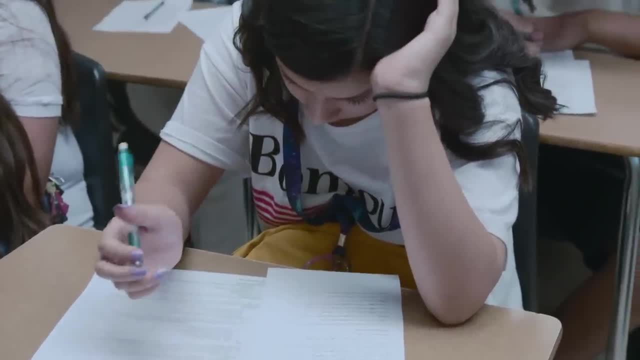 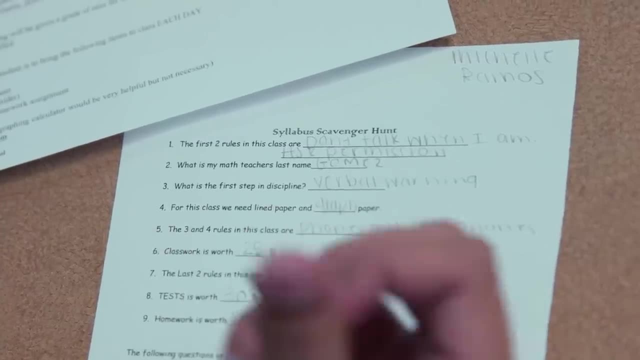 following I actually I think that it's more important to get a printout. they had to do something with it, so it wasn't like they're just hearing me talk. for this whole 50 to 55 minutes they had a chance to get a sheet that was called 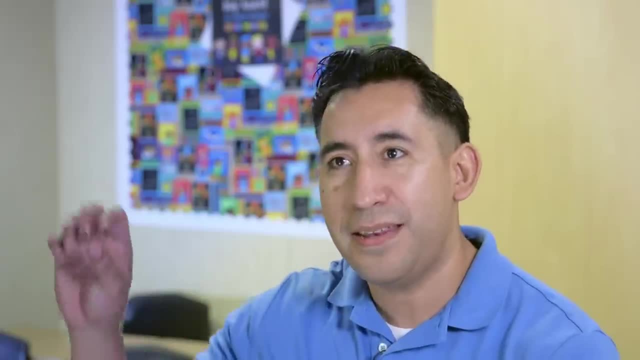 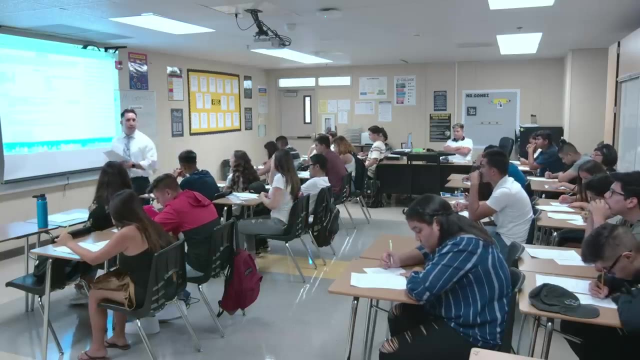 the scavenger hunt and they had to find the answers in the syllabus. before we go over this, really fast, right, just really quick, just so that you know little know a little bit about myself. okay, my name is mr Gomez, obviously, right, it's on your schedule, should be on your schedule, right and at. 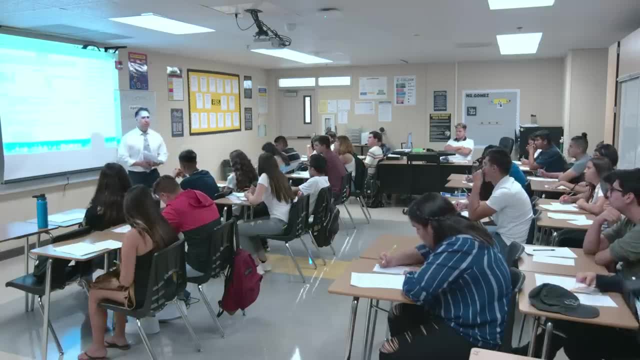 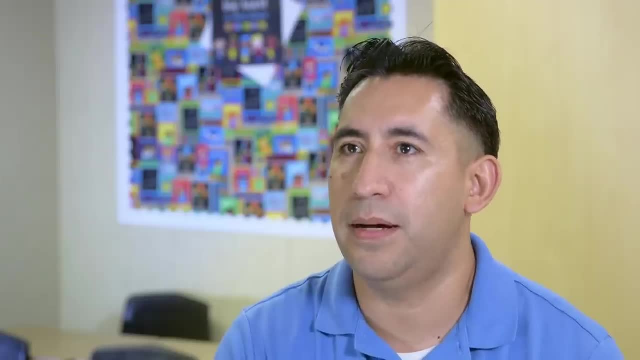 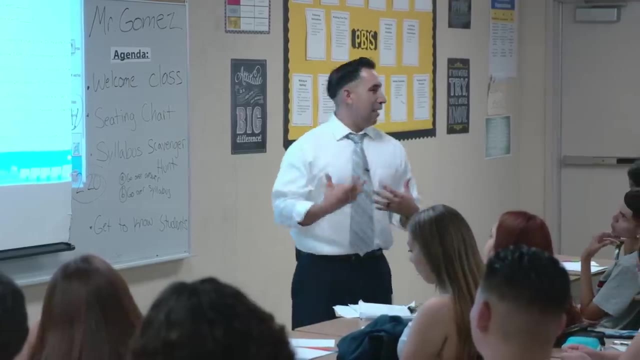 the end it has a letter. what, though? in my name, a Z, I do a lot of telling stories, especially in the beginning of day one, day two. I want them to understand that I am human. it's important for them to see that I did struggle. we have that option to do it, though. okay, I don't think you.